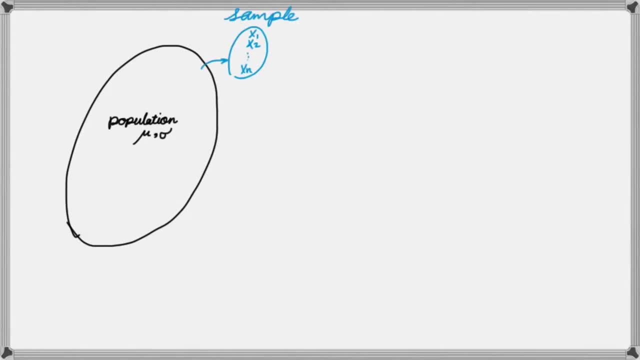 given. Now, if I take a sample from this population, each numerical value in this sample or dataset is the observed value of a random variable that we are interested in regarding that population. For example, suppose that the population is the population of Cal Poly Pomona students and we are 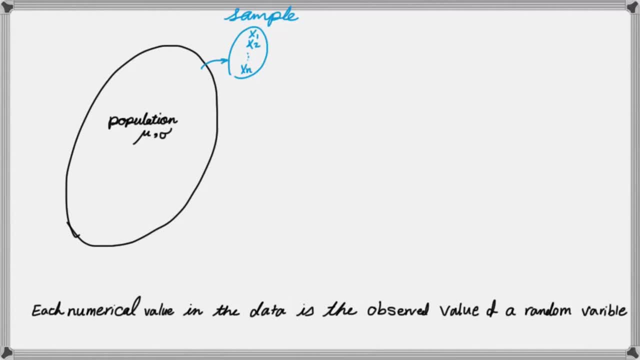 interested in looking into their GPA and I take a sample of n students and look at their GPA values and record that as my sample. Now suppose that I calculate the X bar, which is the average standard, deviation or variance, and the percentage in the sample that I have collected. These values are called statistics. 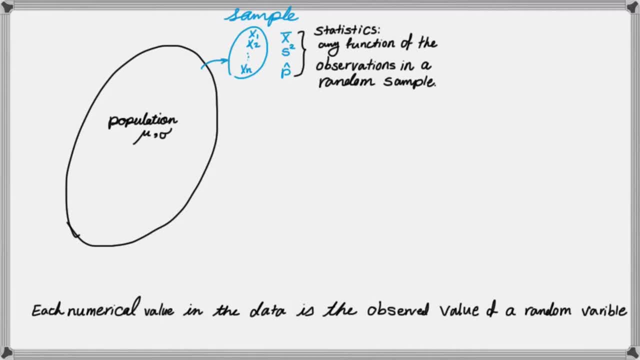 The definition of statistics is any function of the observations in a random sample, because this time we are not looking at the actual observation, We are looking at the function over these observations. Now, if I repeat the sampling process again and every time, calculate the value of these statistics and in the 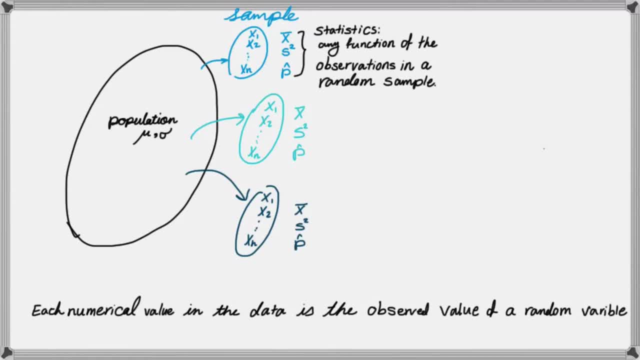 end, look at the distribution of these statistics. we call it sampling distribution. So every time that you are looking into probability distribution of a statistic as opposed to the original data, we call the distribution a sampling distribution. For example, in this case you can look at the histogram of: 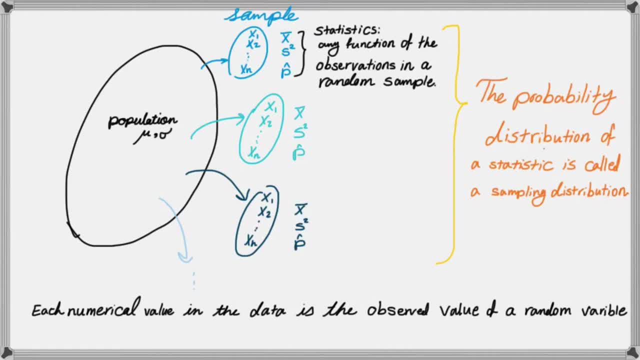 X bar and see what type of distribution you see. or you can take a look at the histogram of variances of the sample or percentage. So, for example, for the percentage, you can look into the percentage of people who got a GPA greater than 3.0 and then 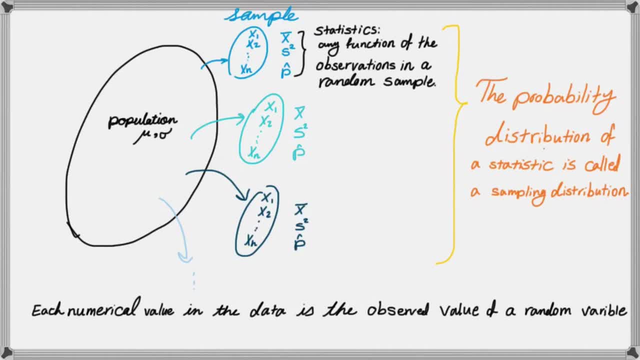 create a histogram for the percentages that you see from each sample. So in this case, we are looking at the histogram of the function that has been calculated over a random sample instead of the actual data that we have collected in the sample. So that would be the definition of a sampling distribution. Also, we talked 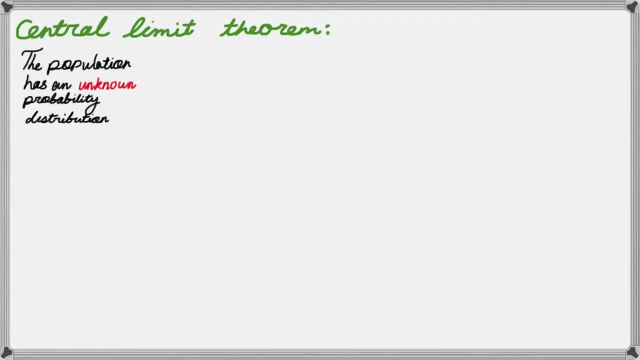 about the central limit theorem. So in the central limit theorem the population has an unknown probability distribution. So basically you can have any probability distribution for your actual population. Of course when we talk about the distribution we are interested in some specific random variable in that population. Again we 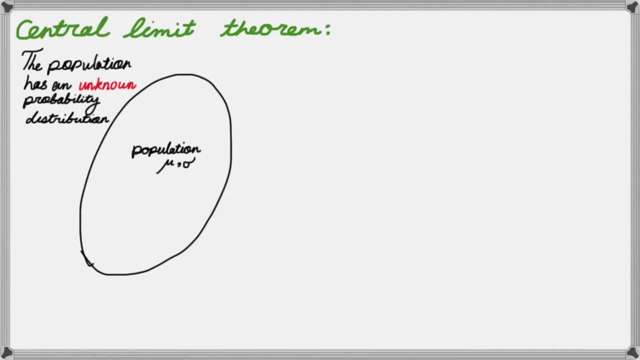 can go back to the example of GPA and suppose that we don't know what the distribution of GPA and K is. But let's say we know what the mu and sigma are. What is the actual population average and standard deviation are? Now, if I repeat the sampling, 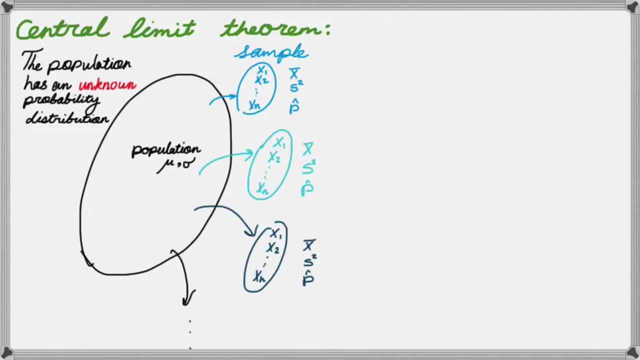 process and look at the histogram of X bar, I can see that it is normally distributed Basically. I can see that bell shaped curve that identifies normal distribution. So the sampling distribution of a sample average or sample mean will be approximately normal, with average of mu and standard deviation of. 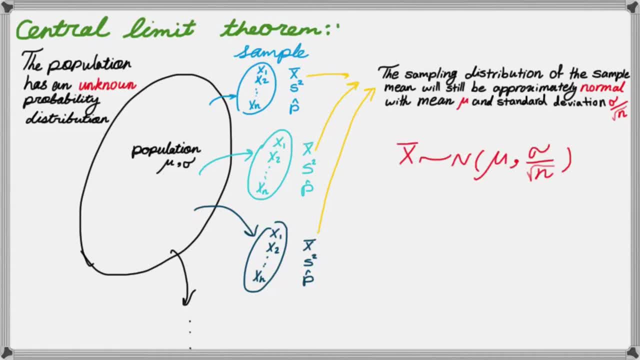 sigma over square root of n. This statement can be summarized like this: So if you keep repeating the sampling process and every time record your X bar and in the end look at the histogram of X bar, you can see that it is normally distributed And it is centered at the center of your. 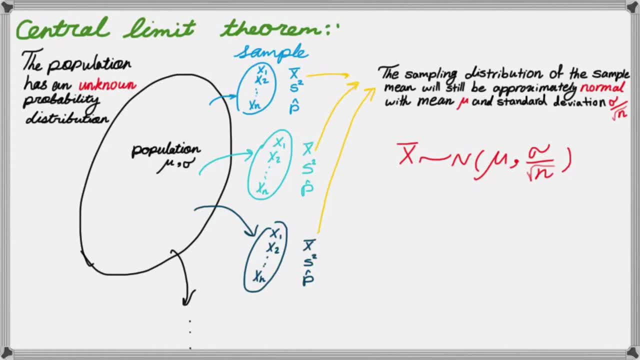 population average and standard deviation is dependent to the sample size, Which will be the population standard deviation over square root of n, where n is your sample size. So this is a very, very important theorem because it says, regardless of your original population distribution, you are always going to have a. 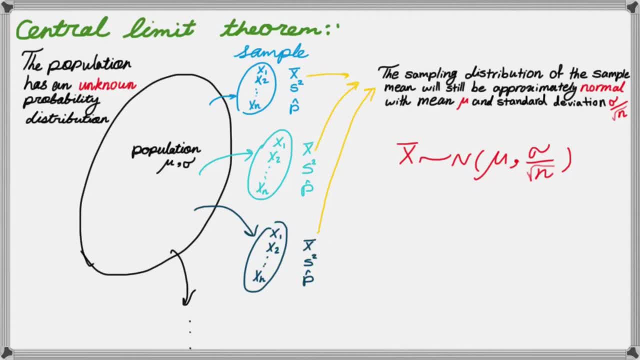 normal distribution. if you look at the distribution of samples that are taken from a normal distribution, This definition and this theory becomes the basis of all the things that we learn after this, including confidence interval, hypothesis testing and so forth, So this is a very important theorem that I expect. 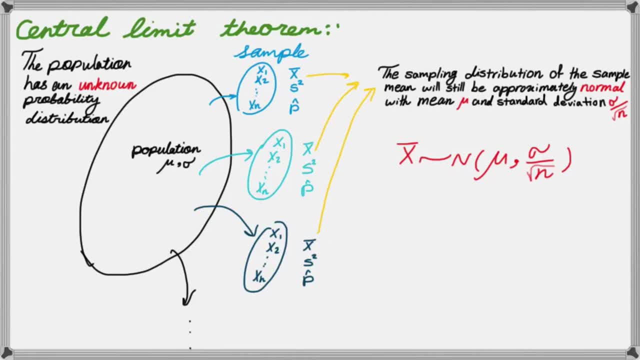 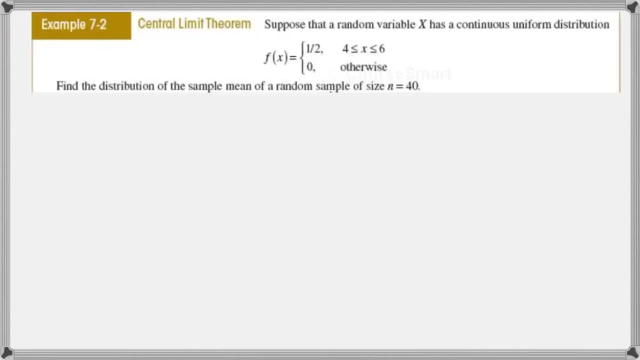 anybody who finished the statistics class carry on to the preceding classes. As your sample size grows to infinity, this normal distribution turns into a standard normal distribution, which is centered at 0 and has a standard deviation of 1.. Now let's look at one example here, which is example 7.2. 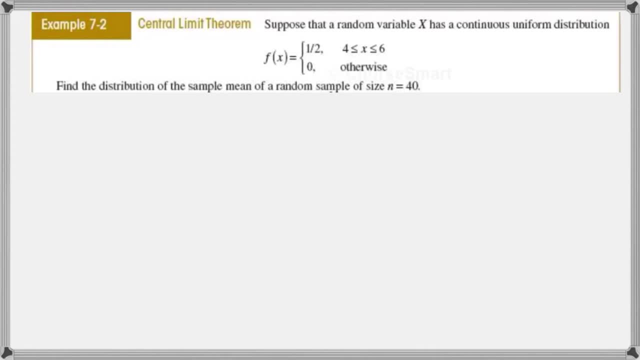 of a statistics textbook by Montgomery. So it says: suppose that a random variable X has a continuous uniform distribution. Find a distribution of sample mean of a random sample of n equal to 40. So it's interested in the distribution of sample average, because you already have the distribution of your X. So now 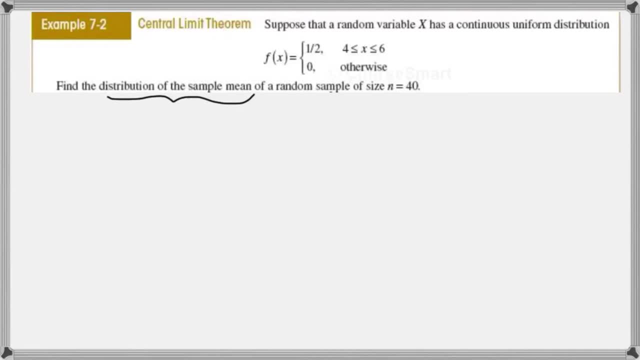 we are interested to know what the distribution of X bar is According to central limit theorem. we know that X bar is distributed normally with average of mu and standard deviation of sigma over square root of n, And mu is your population average and sigma is your population standard deviation. So how we can calculate. 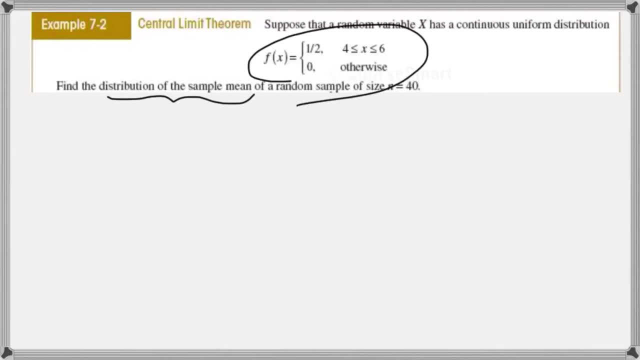 that We know that the population here is distributed according to a uniform distribution so we can calculate its expected value and standard deviation from the definition of uniform distribution. So if I write X is uniform between a and b, we know that the expected value is a plus b divided by. 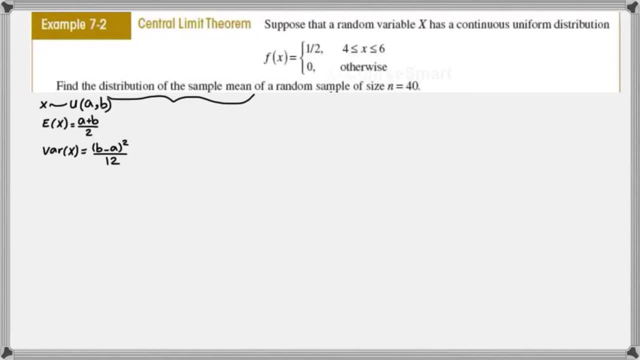 2 and variance is b minus a squared divided by 12.. So now let's replace these numbers. Our distribution right now is uniformly distributed between 4 and 6.. So that means your a and b are 4 and 6.. Now I replace it in expected value definition or. 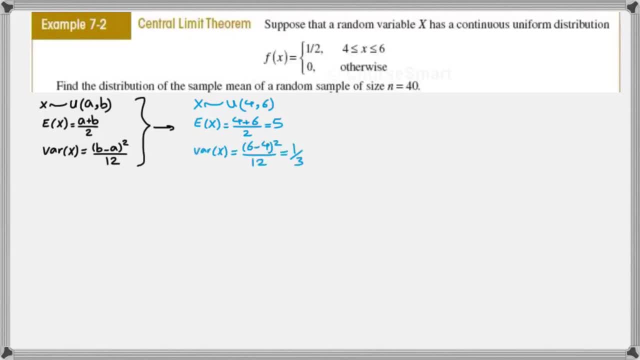 equation and I get 5. And in variance equation I get 1. third. Now this can be my mu and this is my sigma squared, because these are from the actual or initial population. Now, if I show this on a graph, you know that between 4 to 6 we have a height of 1 half. 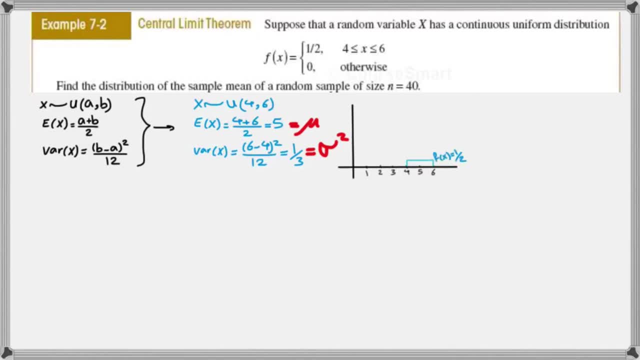 that's why your f is 1 half, And how this 1 half is calculated is basically based on the idea that the area inside this box should be 100% or equal to 1.. We know the base of the rectangular shape is 2.. 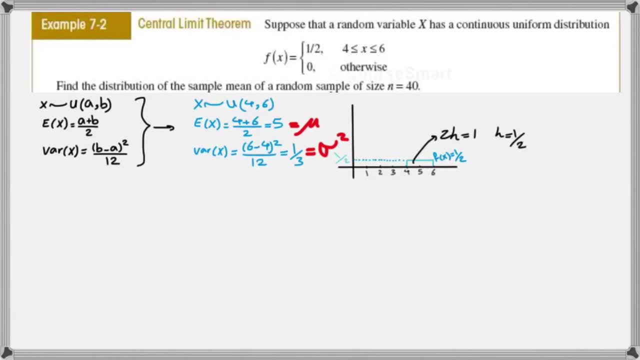 So 2 multiplied by the height is equal to 1. therefore, your height is 1 half. That's where that 1 half has come from. Now that I have this information, I can use the central limit theorem definition for the sample size of 40 and calculate the. 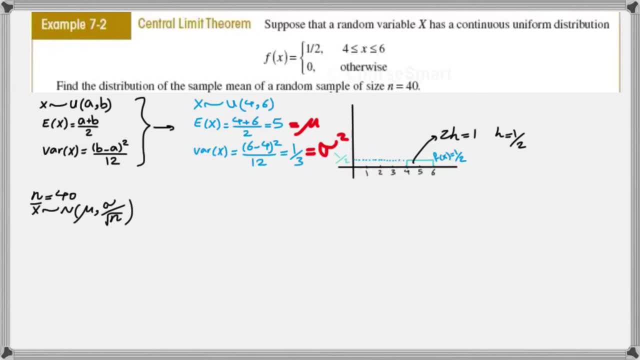 sampling distribution for the sample average. So we know x bar is normally distributed with mu and sigma over square root of n And you always can write this definition regardless of your original population distribution. So if I write x bar is normally distributed, mu is 5 and sigma is: 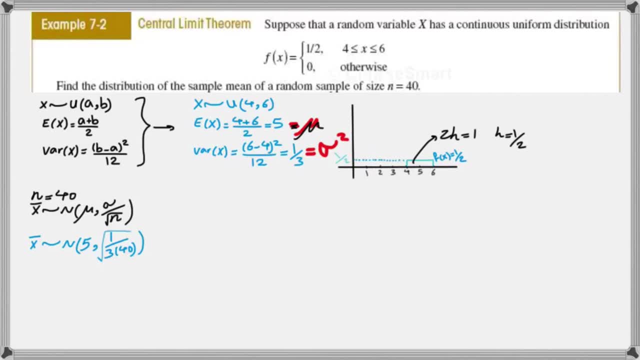 square root of 1 third, because 1 third is your variance And you have to divide it by square root of n, which is square root of 40. So, in summary, you get x bar normally distributed with average of 5 and standard deviation of square root of 1 over. 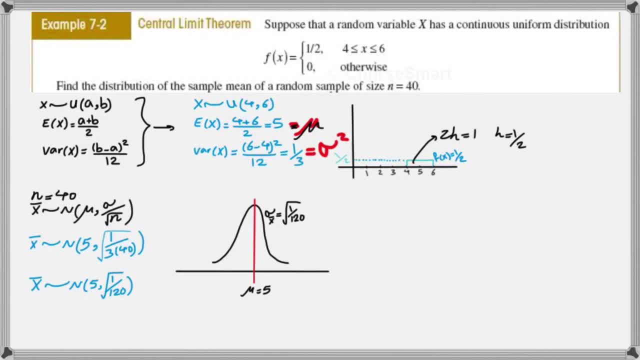 120.. Now what does that mean? That means your normal distribution is centered at 5 and has a standard deviation of square root of 1 over 120.. Now what is the benefit of that? Now you can calculate any probability using the x bar. So if I ask, what is the probability that the sample